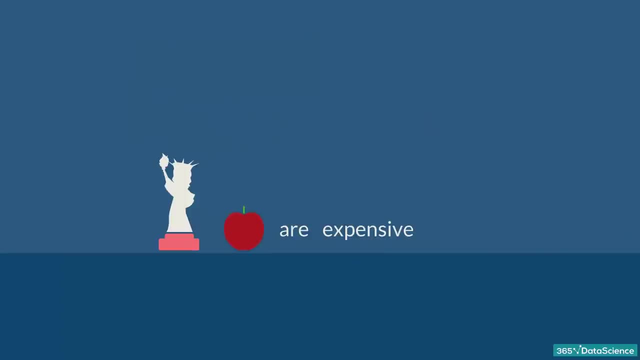 So if I tell you that apples in New York are expensive, this is an idea or a statement, but is not testable until I have something to compare it with. For instance, if I define expensive as any price higher than $1.75 per pound. 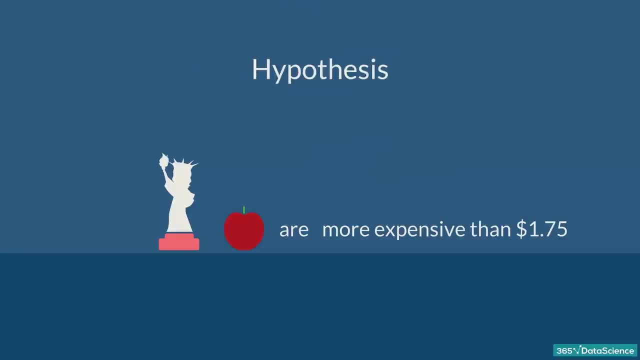 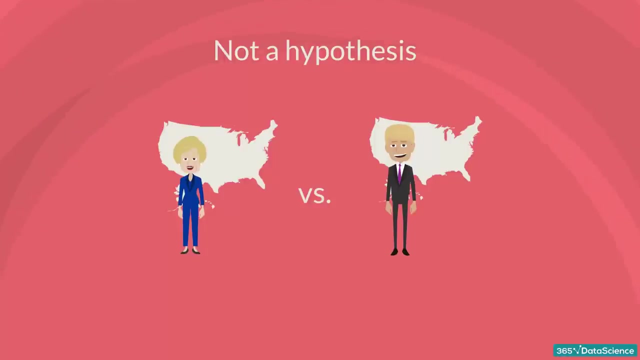 then it immediately becomes a hypothesis. Alright, what's something that cannot be tested with a hypothesis? An example may be: Would the USA do better or worse under a Clinton administration compared to a Trump administration? Statistically speaking, this is an idea, but there is no data to test it. 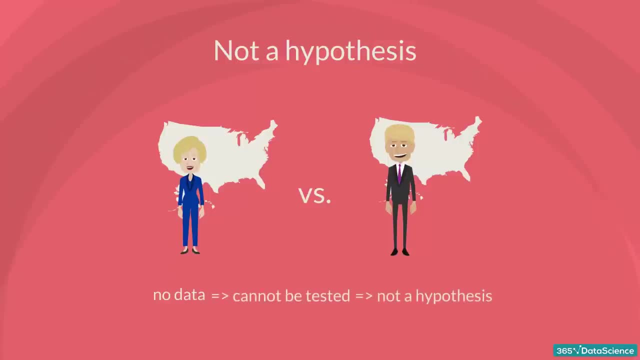 Therefore, it cannot be a hypothesis of a statistical test. Actually, it is more likely to be a topic of another discipline. Conversely, in statistics we may compare different US presidencies that have already been completed, such as the Obama administration and the Bush administration. 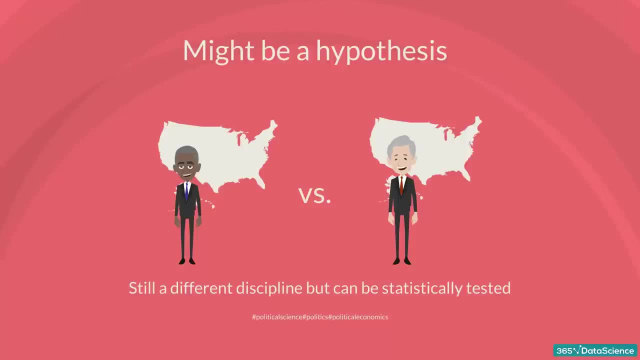 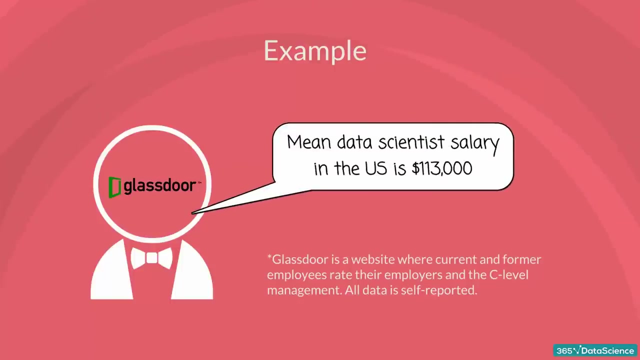 as we have data on both. Alright, let's get out of politics and get into hypotheses. Here's a simple topic that can be tested. According to Glassdoor, the popular salary information website, the mean data scientist salary in the US is $113,000. 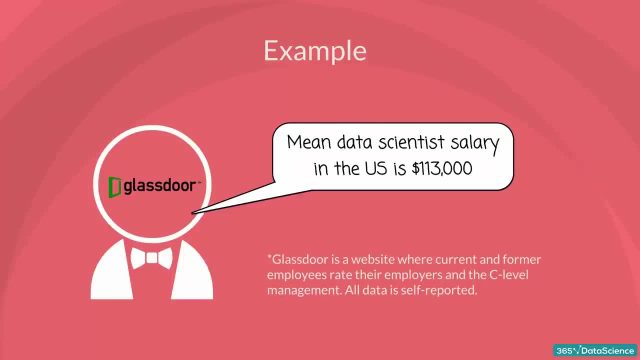 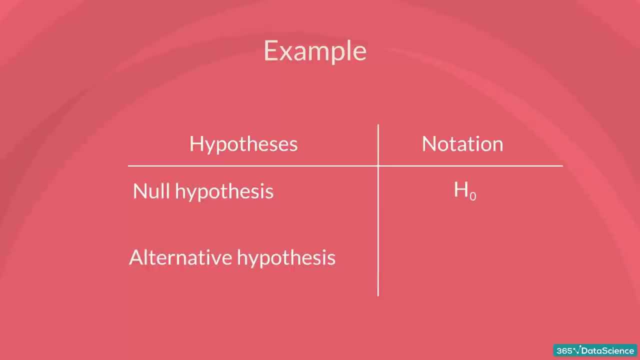 So they want to test if their estimate is correct. There are two hypotheses that are made: the null hypothesis, denoted H0, and the alternative hypothesis, denoted H1 or HA. The null hypothesis is the one to be tested. 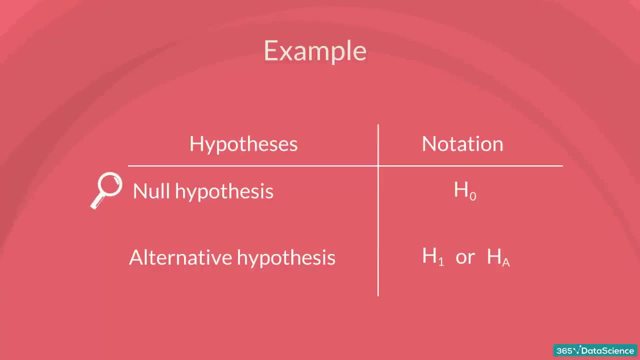 and the alternative is everything else. In our example, the null hypothesis would be the mean data scientist salary is $113,000, while the alternative, the mean data scientist salary, is not $113,000.. Now you would want to check if $113,000 is close enough to the true mean. 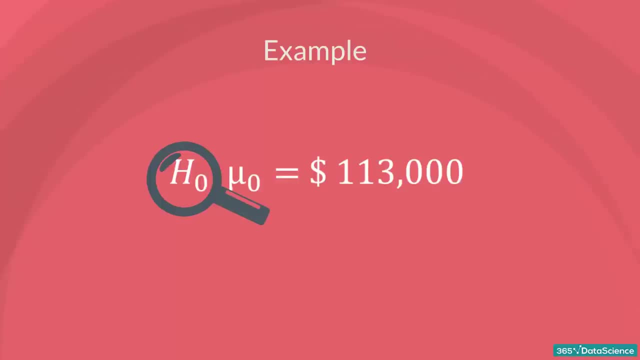 predicted by our sample. In case it is, you would accept the null hypothesis. Otherwise, you would reject the null hypothesis. The concept of the null hypothesis is similar to innocent until proven guilty. We assume that the mean salary is $113,000,. 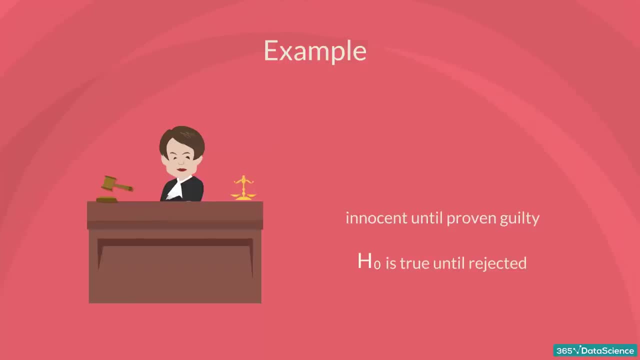 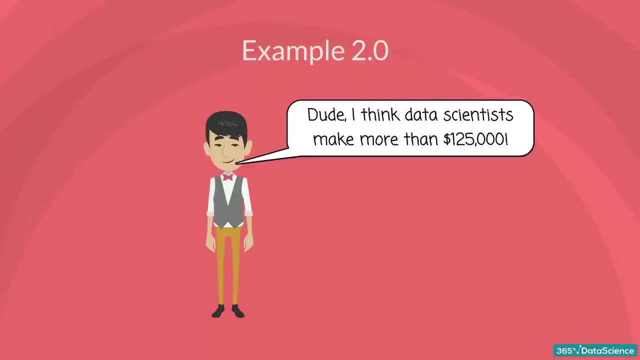 and we try to prove otherwise. Alright, this was an example of a two-sided or a two-tailed test. You can also form one-sided or one-tailed tests. Say, your friend Paul told you that he thinks data scientists earn more than $125,000 per year.